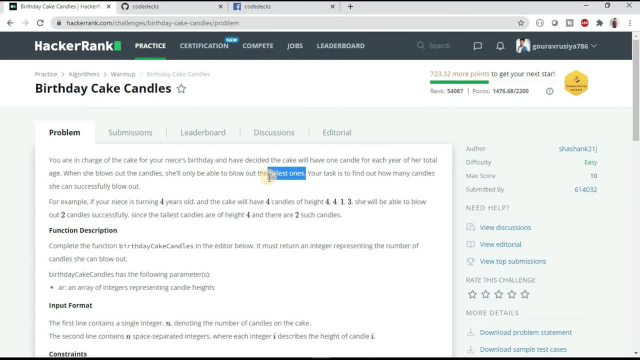 able to blow out the tallest ones. So this is the main task which is given in the problem description. Your task is to find out how many candles she can successfully blow out. So task one is this: Find the tallest one, and the other task is find out how many. 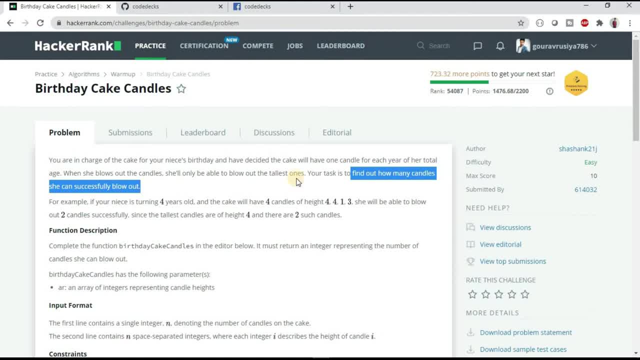 candles she can successfully blow out. That means how many tallest candles are there. The example is: if your niece is turning four year old and the cake will have four candles of height four- one and three, She will be able to blow out two candles successfully, since the tallest candles are of height four And 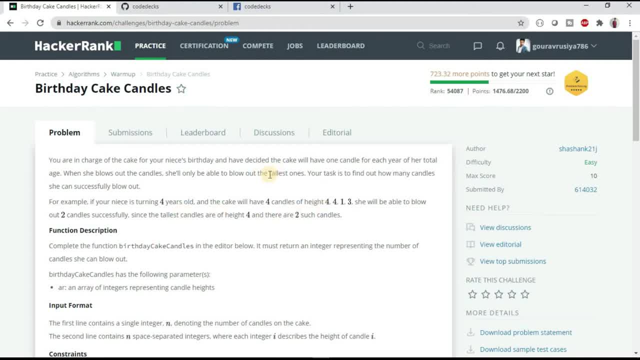 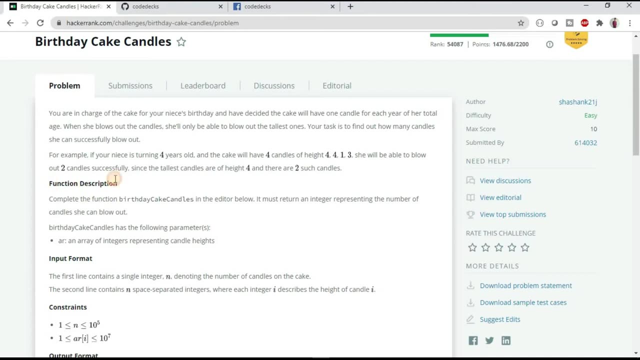 there are two such candles Right. So the first of the task is to find the tallest among all those elements, And the second task is to find out how many of them are tallest. Now let's see how our function should look like. Complete the function. 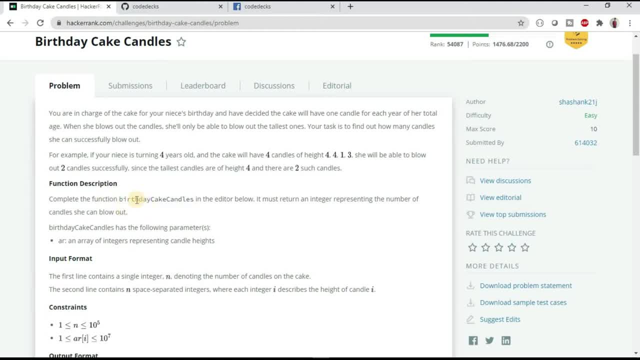 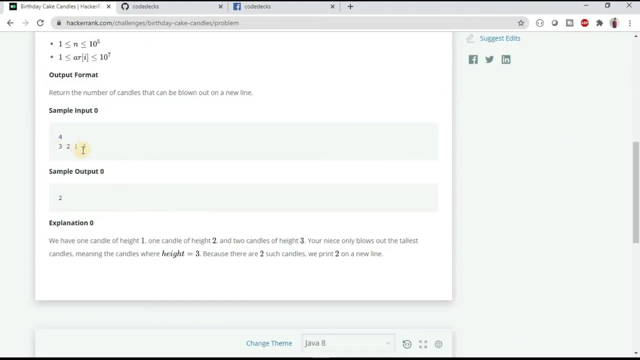 birthday cake candles. so they have given one already written function and we have to write it on the code. inside this method it must return an integer representing the number of candles she can blow out. so this method should return an integer, which is our answer. so for this, 3, 2, 1, 3, you can see tallest is 3 or the highest is 3, and how. 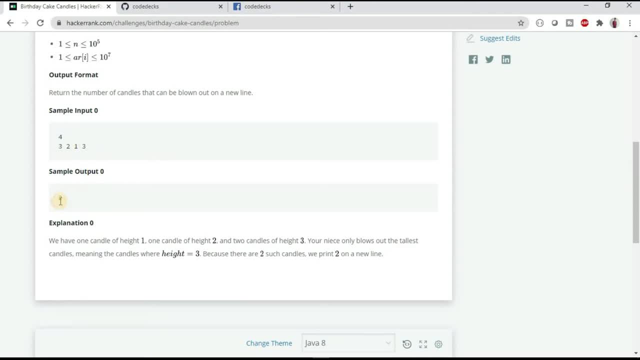 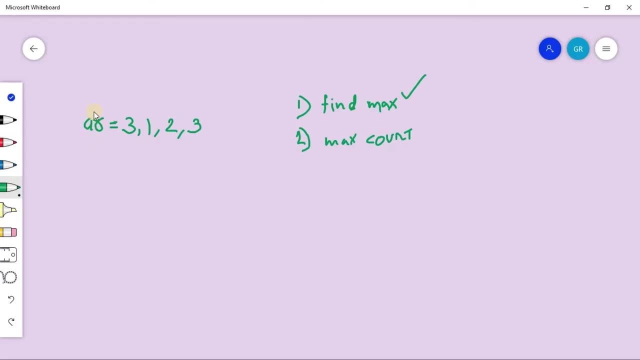 many times. 3, of course, is 2, so you, our solution, should return. let's jump to the whiteboard. so we have given this integer array and these are the candle heights. you have to first find out the max weight. max means, which is which is having the highest height. so here you can clearly see 3. 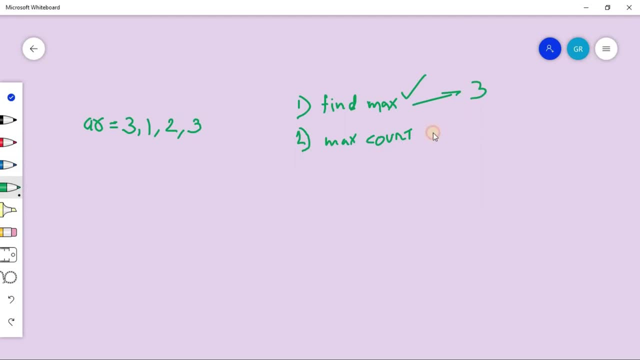 so the max is the highest or the highest. so now we have given this integer which is: so the max is the highest or the highest. so now we have given this integer which will be 3, right, and how many times the 3, 3 came it, it occurs 1 and 2, so it. 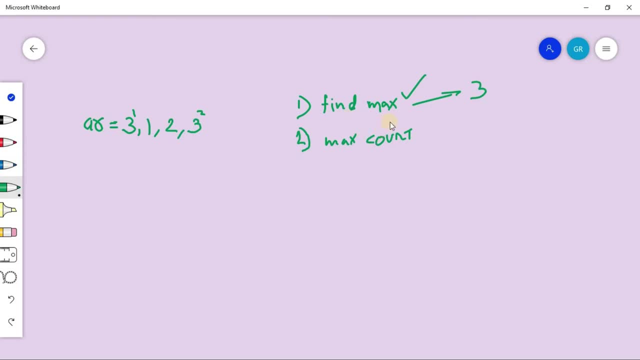 occurs two times now- how we will find the max first. so first what we have to do: once we get the max in in the first for loop, we will again iterate and check. if max is equals to the first zeroth element, then we will check for first. 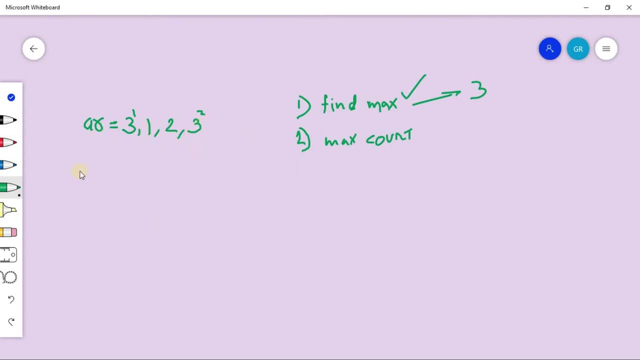 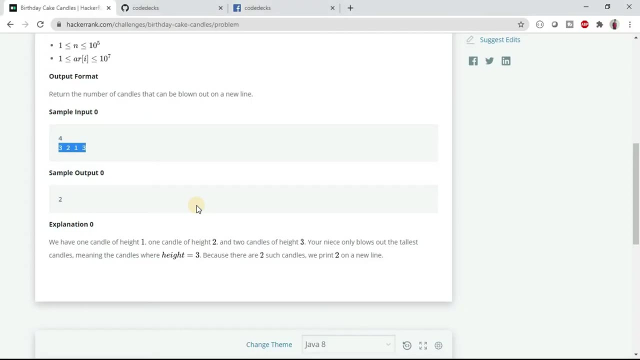 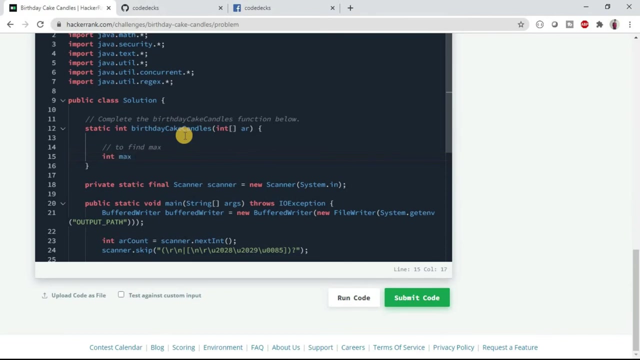 second, third, likewise, for every element, we will check if the max, our max, is equals to any of the element. let's try to jump to solution part of it. so to find max, I will take one integer with which is max right, and we will initialize it with AR of zeroth element. okay, and before this it's good. 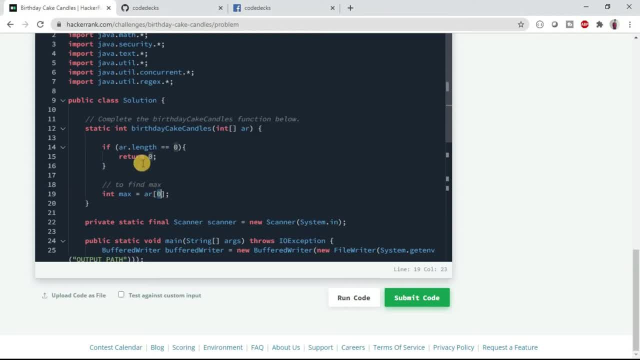 to have this check because we are taking first element from here and if there are no elements, that means length is 0. in that case we are returning 0 from here itself, right? this check is basically for this logic and also it's good to have this edge test here. 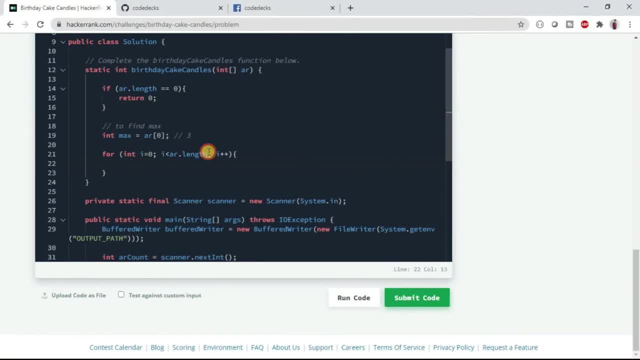 instead of this here, dot length, we can take it as a variable also. here also we will take len and here also we will put the logic inside. this will be if, if, if, whatever there in the max, if it is less than the AR of element, our max will be updated. 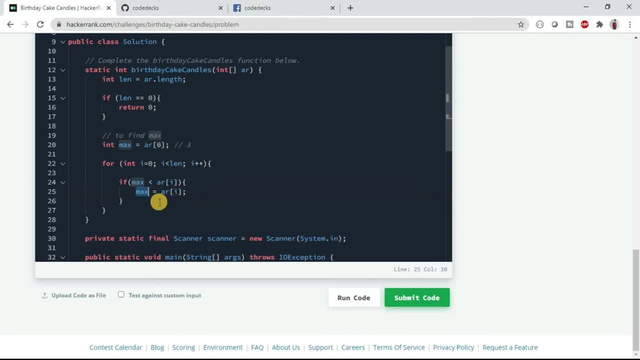 with that value. likewise, our max will always be having the maximum value. so for this example, our max will be 6, right? so with this logic, we found out the max element. now we have to find out how many times this max element came into our array, right, right? so if max value is equals to AR of